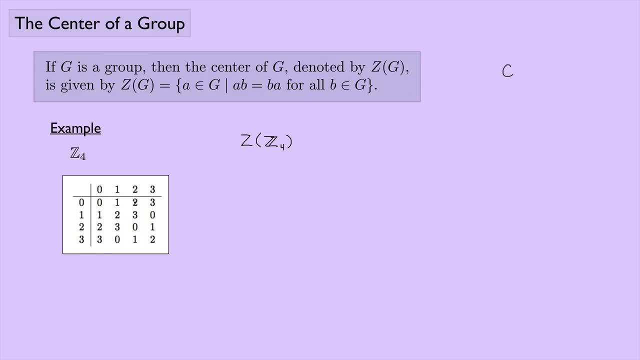 for sure that in this case, zero, which is playing the role of our identity element here, that's going to be in here. So we can say that we know for sure zero is in here. 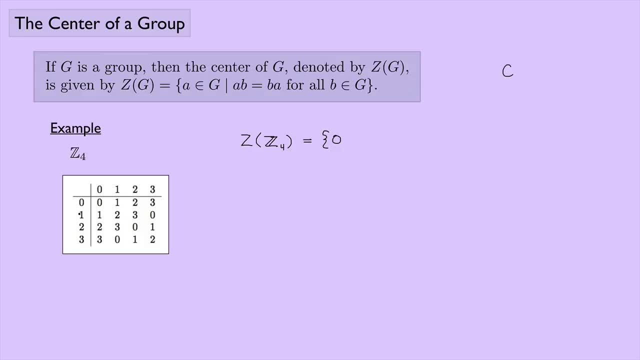 What about one? Well, let's see. One here, it looks like one and two give three, and two and one give three, and one and three give zero, and three and one give zero. So yeah, it looks like one would be in there. How about two? Well, two and one give three, one and two give three, two and three give one, three and two give one. That looks like that commutes with everything. And I think you can check for yourself that three is also in there. So, 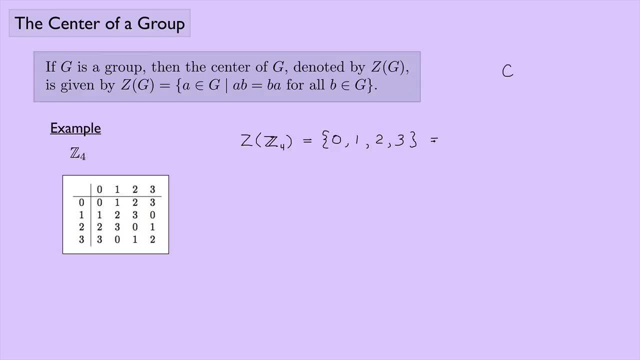 it looks like in this particular case, we just ended up getting the entire group. Now, that's not so unusual here if you think about it. This group here is abelian. That means every element commutes with every other element. So if we happen to have an abelian group, so if we know that G itself is abelian, meaning that every element in G commutes with every other element in G, 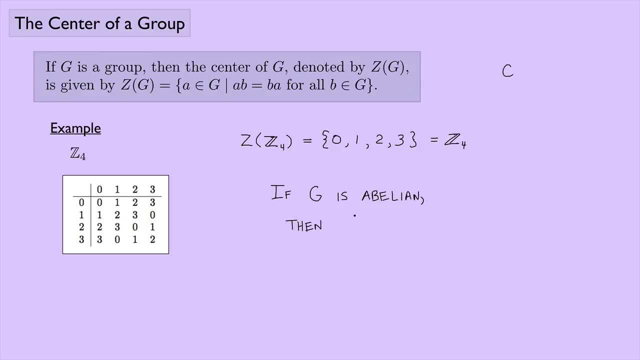 then we can say for sure, that the center of G is going to be just the group itself. So that's not very exciting. Let's see if we can get a more exciting case. Maybe if we try something that's non-abelian. Okay, so here's our 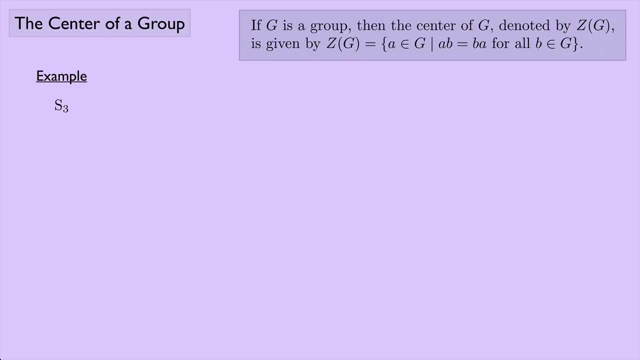 definition of the center of a group. And now let's look at the group S3. If you remember, that's the group of symmetries on an equilateral triangle. Here is the group table for S3. And now we're 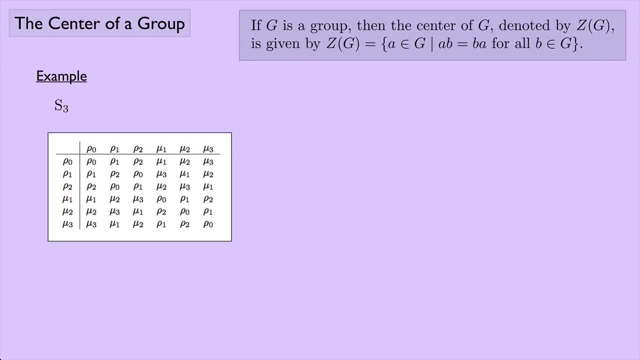 going to try and find the center of S3. So like I said before, it's pretty clear that the identity element, which in this case is rho naught, that's going to be in the center. So if we're looking for the center of S3, we can say for sure, for sure, that we are definitely going to have the identity element. So that would be rho zero. But do we have anything else? So let's look at rho one. So rho one right here. Well, how about rho one and mu one? So if we look at rho one, mu one, we're going to have the identity element. So if we look at rho one, mu one, what do we get? So rho one, starting on the left over here, and then mu one is mu three. All right. And what about mu one rho one? Does that work? So mu one rho one is mu two. So it looks like rho one, no good. How about rho two? Okay, so rho two, let's pick an element here that maybe one of these elements here. How about, well, we can do it again with mu one. How about, does rho two commute with mu one? So rho two and mu one, that gives us mu two. Okay, and what if we do it the other way around? How about rho, or mu one rho two? Does that also give us mu two? So mu one rho two, nope, that gives us mu three. So it looks like rho two, no good. Okay, well, we didn't have any mu's. How about the mu's? Maybe the mu's will work. Well, we just saw that mu one and rho one, it didn't commute. They didn't commute here. So we know mu one can't be in the center here. 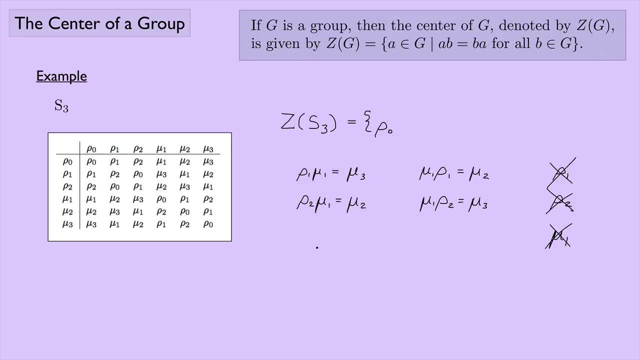 So mu one, no good. How about mu two? So let's try mu two together with about rho one. 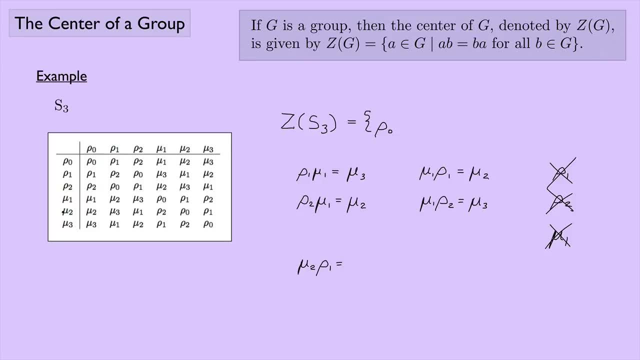 Well, we kind of know that this probably shouldn't work, let's check it anyways. So we have mu two and rho one, that gives mu three. And what about rho one 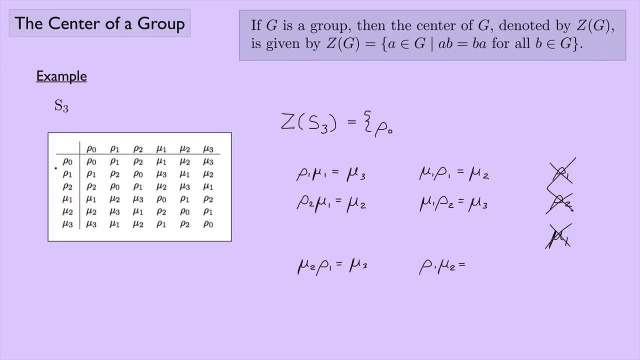 with mu two? Does that work? Rho one with mu two, that's mu one. So nope, mu two, no good. 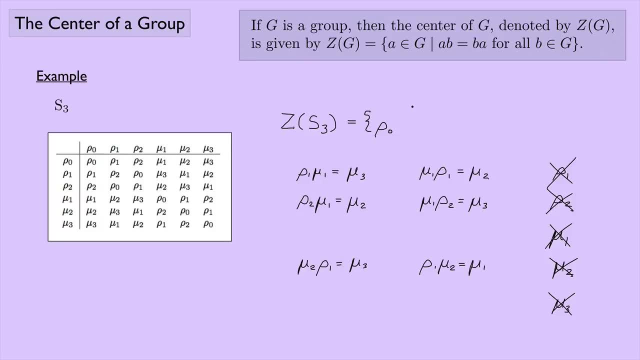 And you can check for yourself, mu three, that's also no good. So that's it. Our center, well, that's just the identity element. That's not very exciting. So, it looks like when we have an abelian group, we have the center as the entire group. 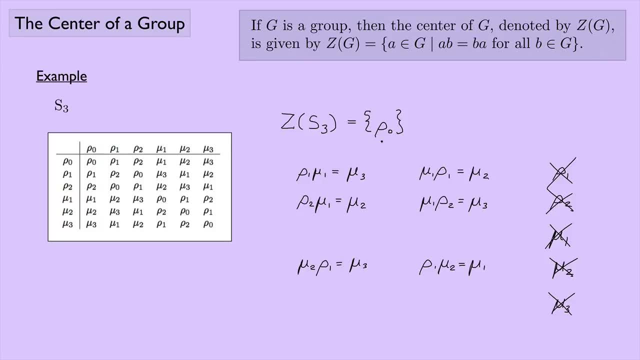 We just saw an example where we have a non-abelian group and the center was just the identity element. Is it possible to have the center be anything other than the entire group or just the identity element? Let's look at one more example. Let's look at d four. So this was the 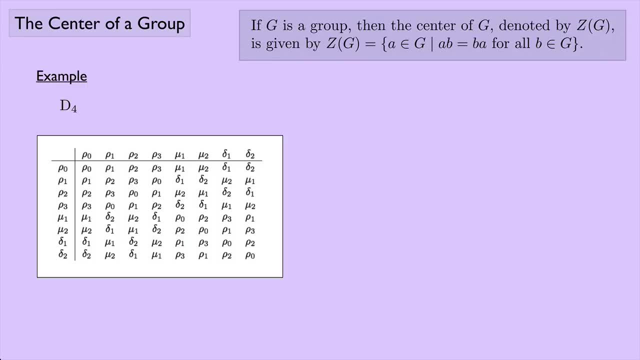 group of symmetries on a square. So here's the group table for d four. And we're going to try the center of d four. So the center of d four, z of d four. Okay. So we know for sure we have the identity element, which was rho zero for this group. But do we have anything else? So let's see here. Well, let's try rho one. So how about rho one and mu one? So what does that give us? So rho 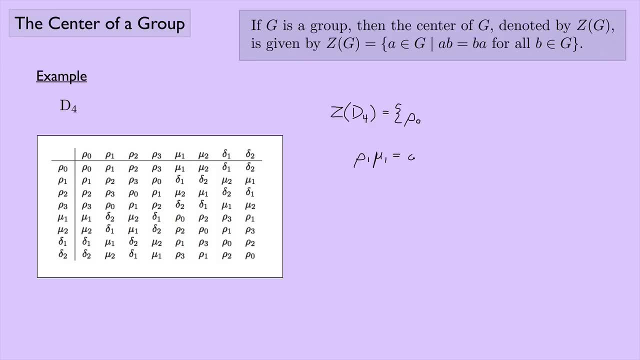 one, mu one, that's delta one. Okay. And then how about the center of d four? So the center of d four, 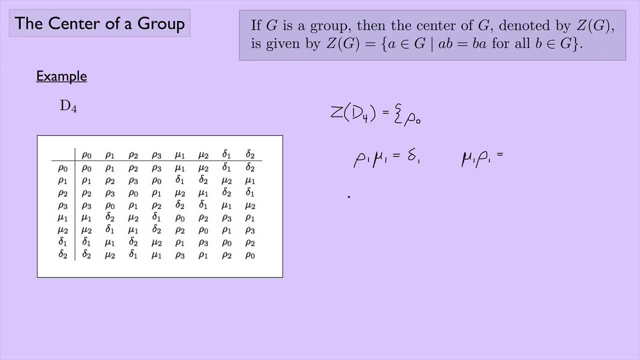 mu one, rho one. So let's see if rho one commutes with mu one. So now we have mu one, rho one, that's delta two. No good. So we can see rho one. Nope, not in the center. How about rho two? So let's see. How about rho two? Well, let's kind of look at the rows here, at least here. And rho one and rho two is rho three. Well, that seems to work. How about rho two and rho three? So rho two and rho three give rho one. And rho three and rho two give rho one. This is looking promising. Okay. Let's do an example here, looking at the one of the mus. How about rho two and mu one? So rho two and mu one, that's mu two. All right. And now let's try it the other way. Row one, I'm sorry, mu one and rho two. And is that going to give us mu two? Let's check. Mu one and rho two, it gives us mu two. All right. This is looking good. So if you go through the rest of these, I won't write them all out here, but we'll kind of look at the group table. Rho two and mu two is mu one. Mu two and rho two, that's also mu one. 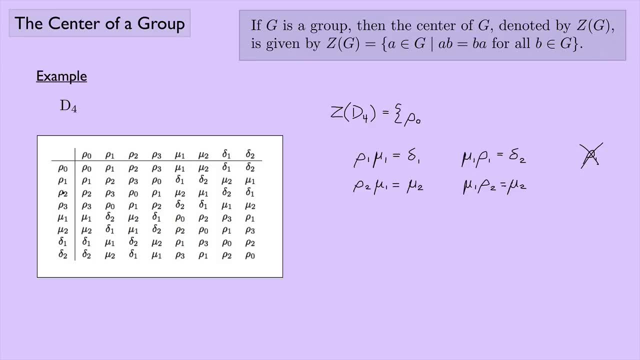 And then if we look at rho two with the deltas, rho two and delta one is delta two. And delta one and rho two is also delta two. And then finally, rho two and delta two is delta one. And delta two, 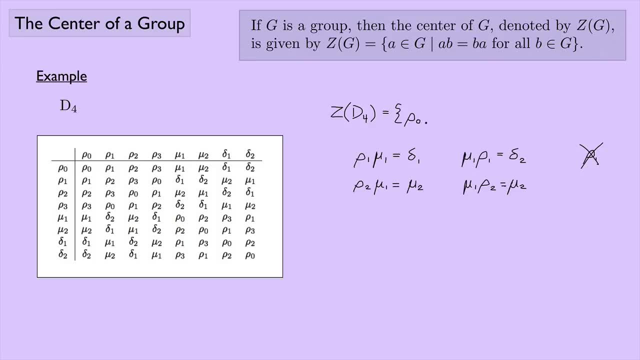 rho two is also delta one. So it looks like we do have another element in this center here. We can say rho two is in there. 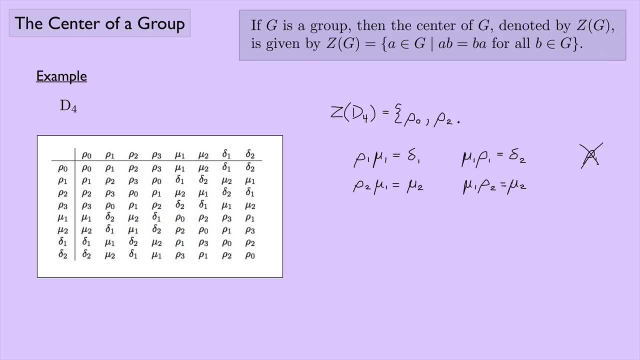 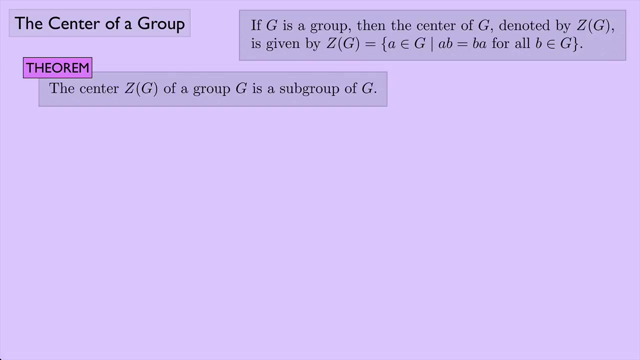 If you go through and you check the rest of these, it turns out nothing else really works. We end up just with these two elements being in the center, but we see that we have a non-trivial center here. So it is possible to get a center that is more than just the identity element or the entire group itself. So it turns out that the center z of g of a group g is a subgroup of g. So if we wanted to actually prove this theorem here, to show that z of g is a subgroup of g, and to show something is a subgroup, we can use the subgroup test. So the subgroup test says a non-empty subset h of a group g is a subgroup of g if and only if the following properties hold. And we have closure and inverses. 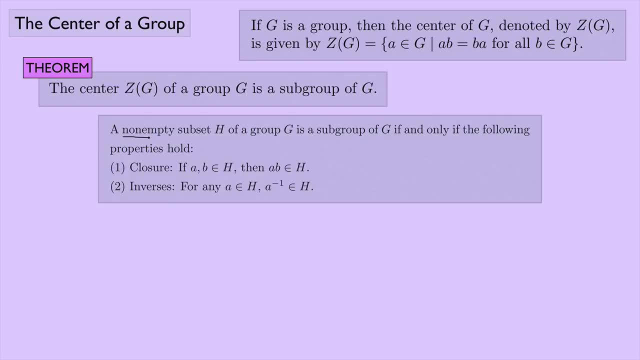 Okay, well one thing right off the bat, we see non-empty subset. Well, we know that the identity element e is definitely going to be inside the center. We saw that already before. So we have something that's non-empty, but now we need to check closure and we need to check inverses. 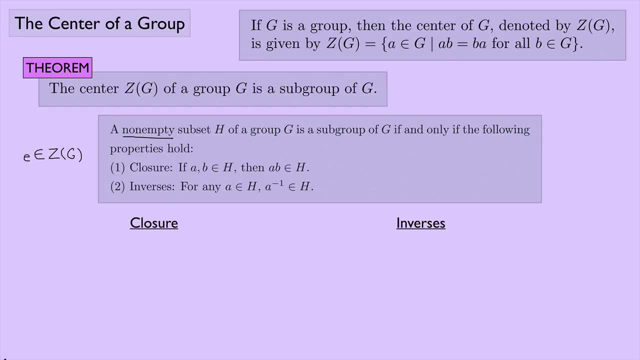 Okay, so let's just do a sketch of a proof here and then I'll do a formal proof. So first let's check closure. What does closure mean? Well, that means that if we take any two elements in the center and we do the binary operation on them, we should get something else that's in the center. So let's pick two elements here. How about x and y? We'll use letters different from the a and the b that we have up here. Let's say those are in the center. And we need to show then, we have to show that x times y is in the center. Okay, so how are we going to show that? Well, we know that these x and y's, if they're in the center, are going to commute with any element that's in g. So if c, say, is some element in g, we know that x times c is c times x, and we know that y times c is c times y. So we need to show that xy times c is c times xy. This is what we have to show right here, this condition. Okay, so how are we going to show that? Well, how about if we use these two properties here, and I can kind of rearrange things here so that I group the y and the c together. So I'm using the associative 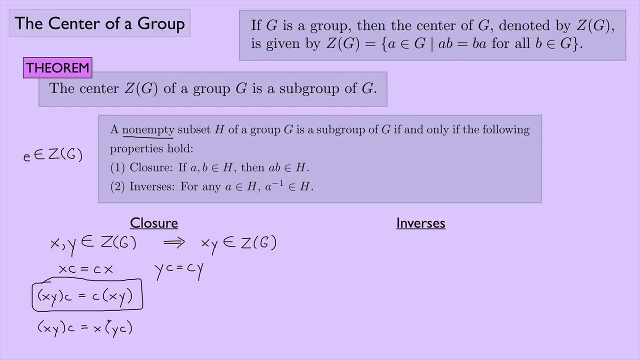 property here, and you might wonder, well, I didn't show that yet. How do I know I can use it? But remember, x, y, and c are all in the group g, and since g is a group, it is associative. So I don't have to worry about that. 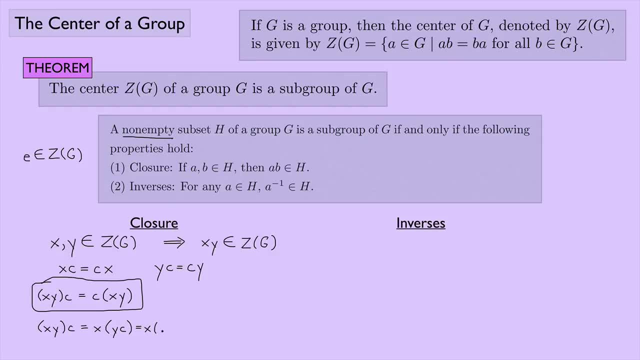 But now I can just kind of move things around here. So the y and the c commute, so I get cy, and then I can kind of change it around, so I group the x and the c together, and then I can change the order of those, and then I'm done. I have c times xy. Great. Okay. 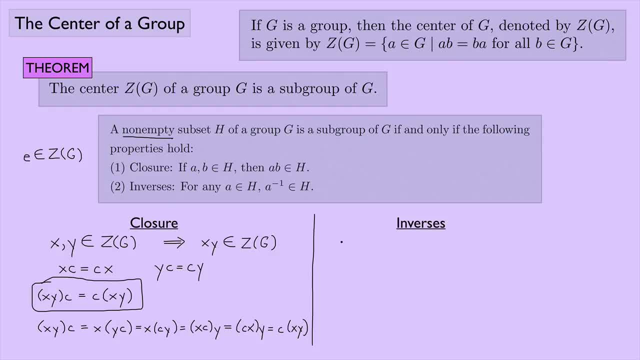 How about inverses? So I have to do a similar thing. If I know that x is some element of the center, I have to show that the inverse of x is also in the center. So x inverse is also in the center. Okay. How am I going to show that? Well, let's see here. I have to show that x inverse is in the center, which means it commutes with every element in g. So again, I'm going to have to use some property that involves an element of g. So let's say c, again, is some element of g. Well, I know that that's true. If x is in the center, then x times c equals c times x. And I also know that if c is in the center, then x times c equals c times x. 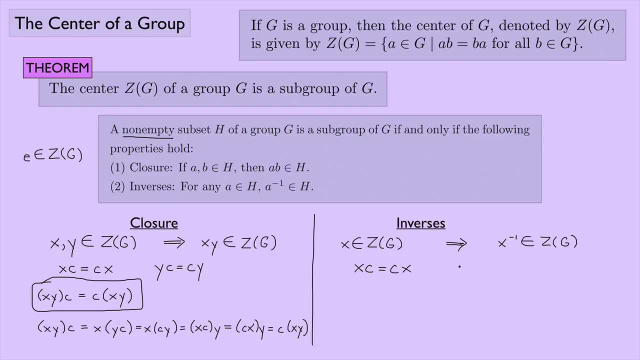 c is in the group g. I know that c inverse is in the group g, which means that I can say that x c inverse equals c inverse x, since x is in the center, commutes with every element, including the inverse of c. Okay. So now I need to show that x inverse and some element c is equal to c x inverse. That's what I have to show. How am I going to do that? Well, let's see. x inverse and c. Well, whenever I see inverses, there's a good trick you can always use. That's using this idea here. If you have a times b inverse, that's the same thing as b inverse a inverse. And that's something that whenever you see any proof involving inverses, there's a good chance something like that's going to come up. So if I can kind of rewrite this to use this idea here, maybe it would work. So how about if I say that this is like x inverse, and this is c inverse inverse. 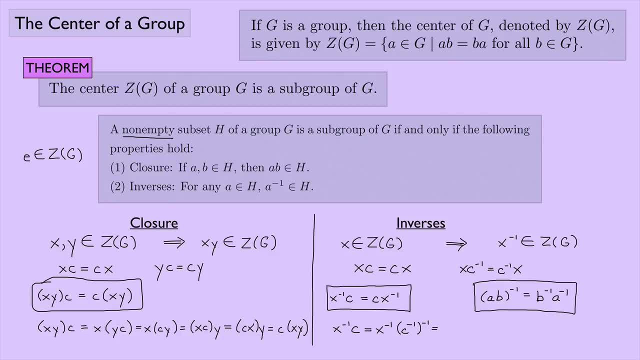 Same thing, right? Now this looks kind of like this. So I can kind of turn it into that. In other words, I can rewrite this so that I have something that looks like c inverse x inverse. And now I'm good to change these around because remember, c inverse x is the same thing as x c inverse. So that's x c inverse, whole thing inverse. And now I can undo this that I was doing here before. And if I do that, then the order switches again, and I get c inverse inverse x inverse. But c inverse inverse is just c. So this is c x inverse. And I'm done. I think it's time for a formal proof. 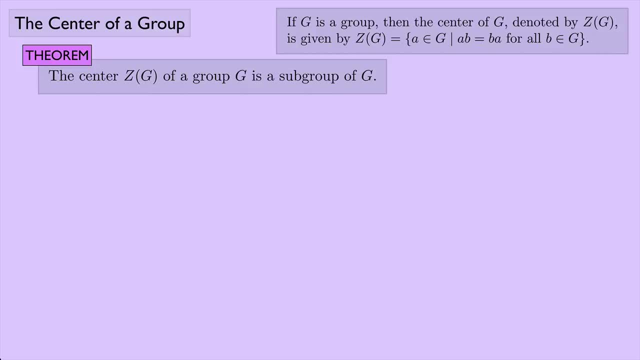 Okay, so for the formal proof here, here's the theorem. The center z of g of a group g is a subgroup of g. And I am first going to note that the identity element that I'm going to denote as e here, I know that e is in the center. So I know that the center is non-empty. So now I'm okay to use the subgroup test. So for the subgroup test, I have to show that the center is closed and that any element of the center also has an inverse in the center. So let's break it down into closure and inverses. So first closure. Let's let x and y be any two elements in the center. And then I know that x times c equals c times x. And y times c equals c times y for any element c that's in g. And that's just going by the definition of what it means to be in the center. So now I can do that thing where I kind of group 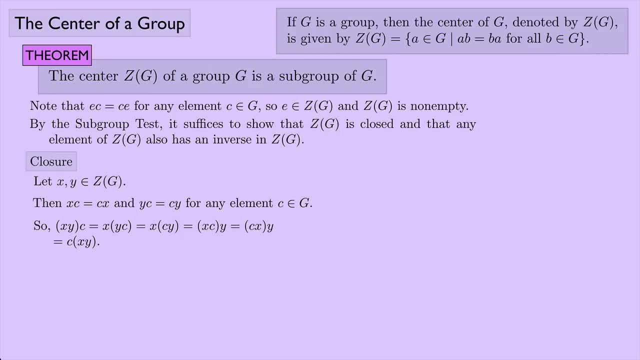 things together. So I get x times y times c. And then I can change the grouping around and change the ordering just like we did before. And if you see, you end up getting c times x times y. So this is great. This is what I want to show. So this implies that x times y is in the center. 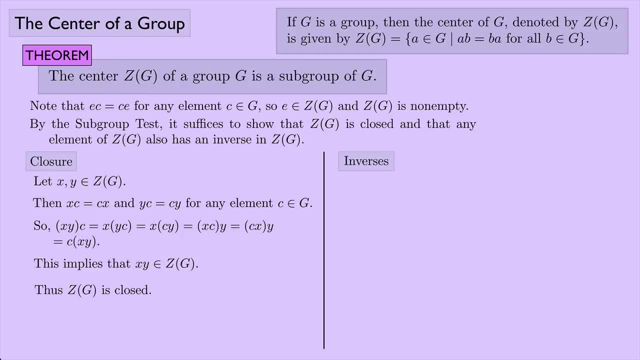 And so the center is closed. So I can do that. And then I can do that. And then I can do that. And the center is closed. Okay. How about inverses? Well, let's let x be an element of the center.